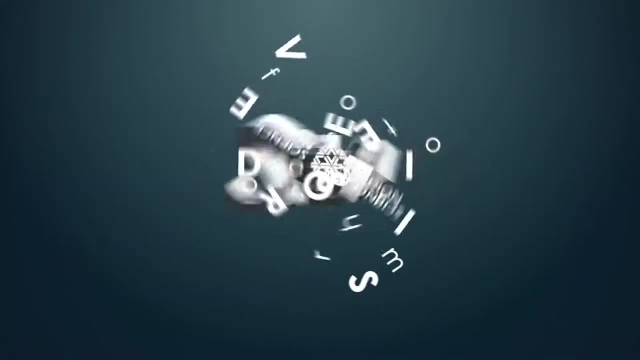 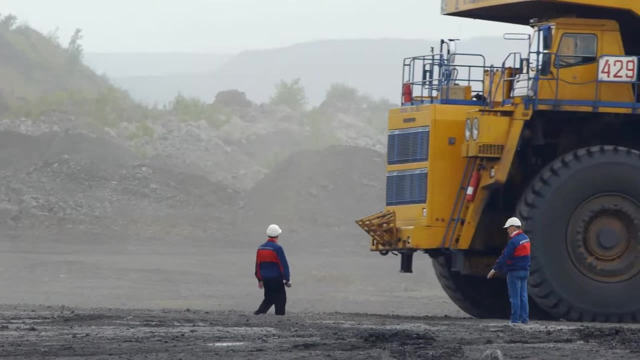 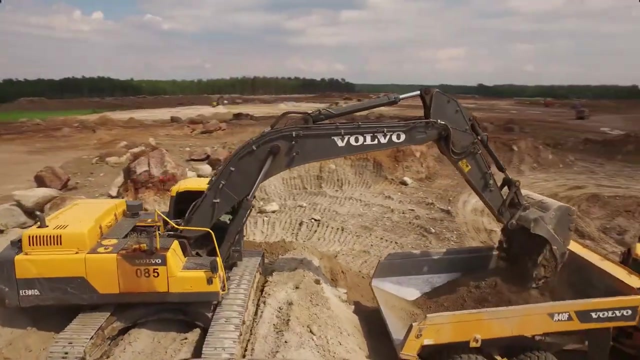 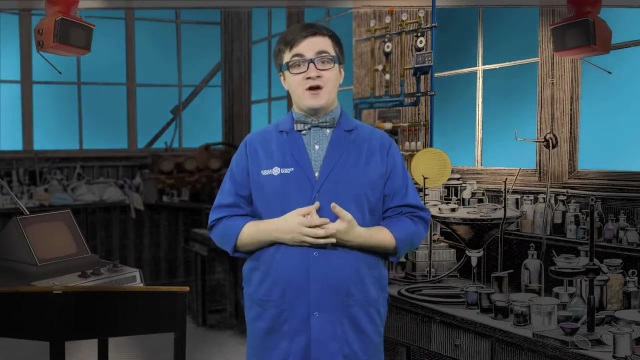 What do you think of when you hear the word machine? A machine is something that makes it easier to do things. Did you know that there are some machines out there that are very simple? They often have no or very few moving parts and no motor. Really, There are six basic 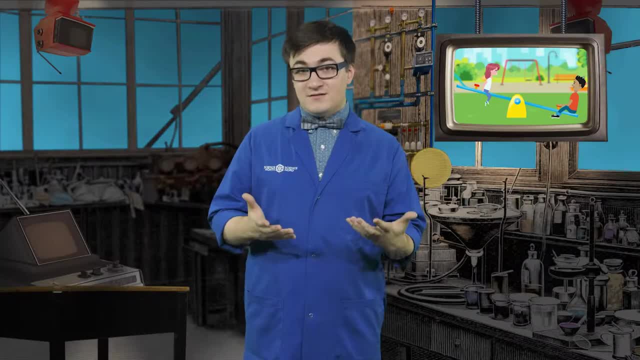 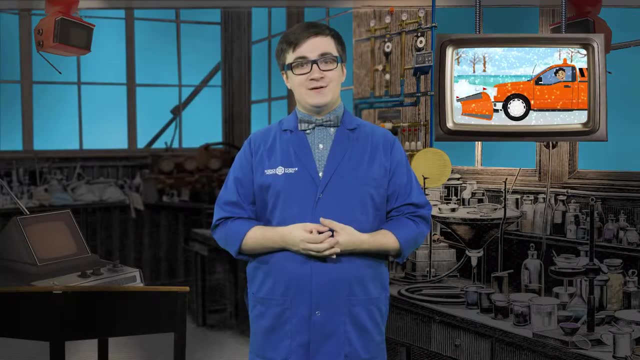 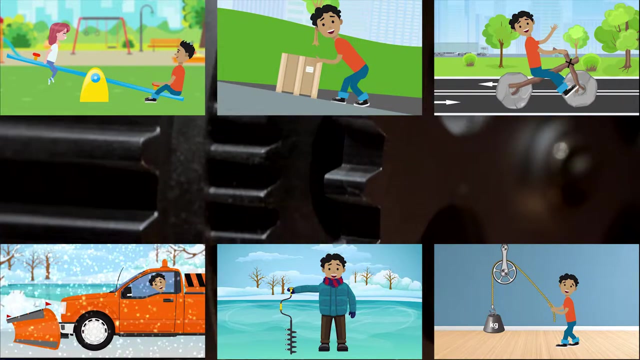 types of simple machines. They are the lever, the inclined plane, the wheel and axle, the pulley, the screw and the wedge. These simple machines make work easier by letting us move things with less force. Levers: let us use less force by having the force act over a greater distance. 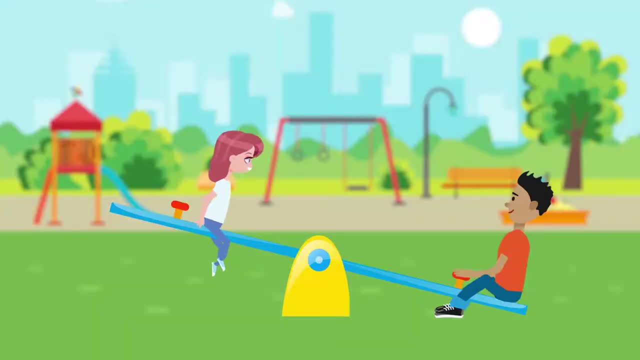 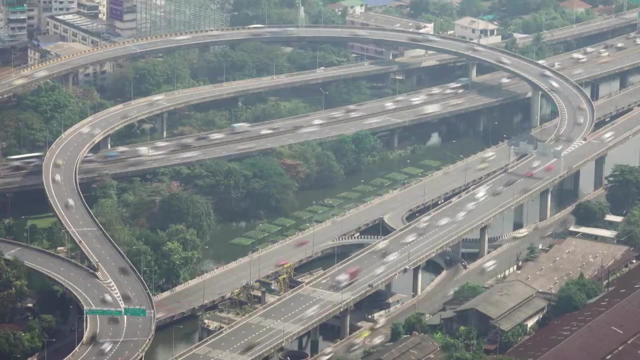 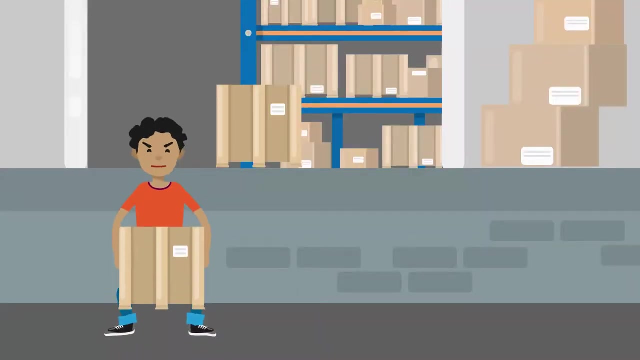 For example, on a seesaw, a smaller person can lift a larger person. if the smaller person moves further away from the pivot point, An inclined plane will spread the force over a greater distance too. Instead of lifting a heavy rock straight up, you can use a ramp to reduce the force needed to lift the rock. 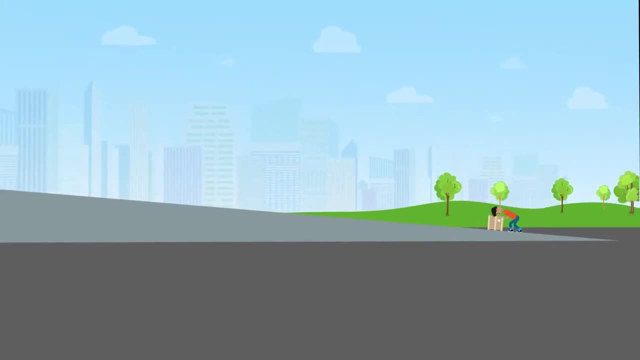 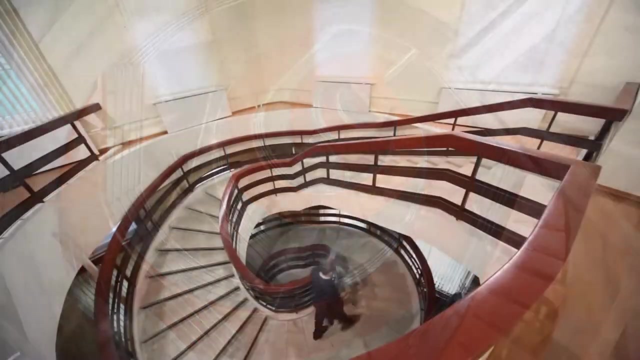 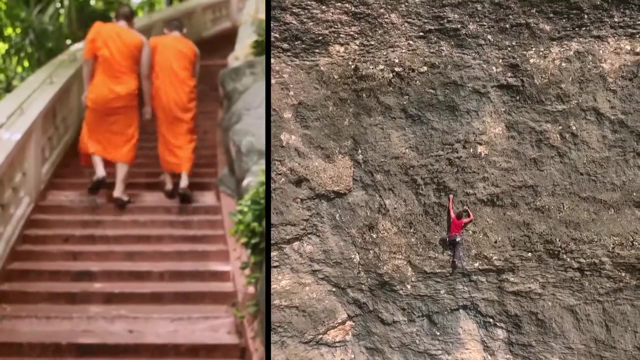 But you need to drag the rock for a longer distance. Sometimes inclined planes do not look like inclined planes. Take, for instance, this: Stairs make it easier for us to go up because the force is spread over a greater distance. Ramps make it even easier for us to go up. Ramps also help people who cannot use stairs. 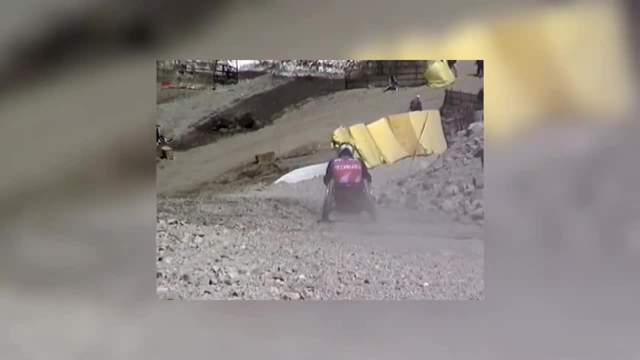 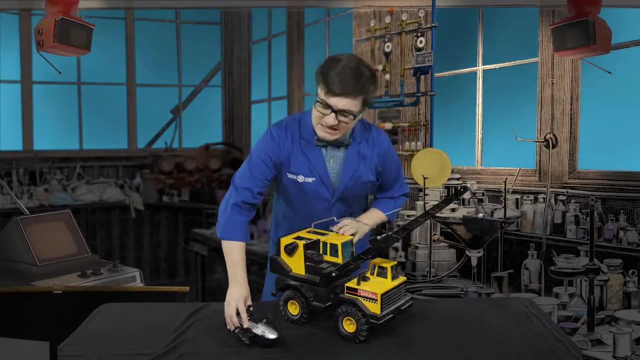 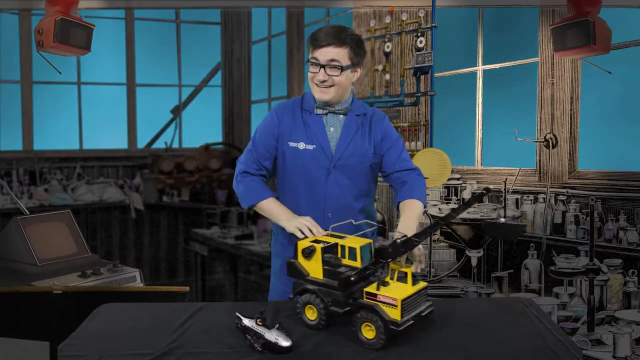 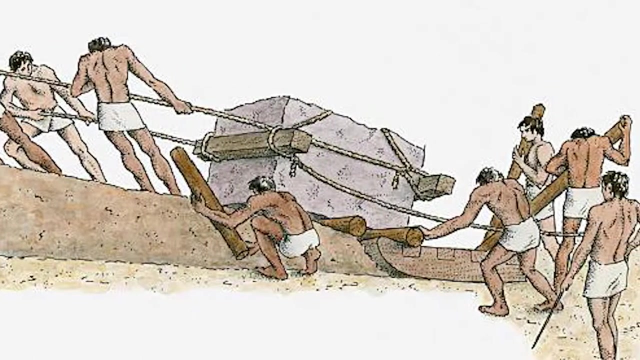 like people in wheelchairs. Speaking of wheels, the wheel and axle make work easier because they reduce friction when you move something. Initially, humans used log rollers or rocks to move things, and they had to take rollers from behind and put them in front. 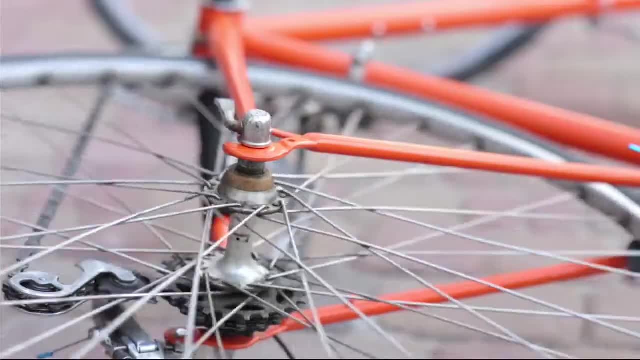 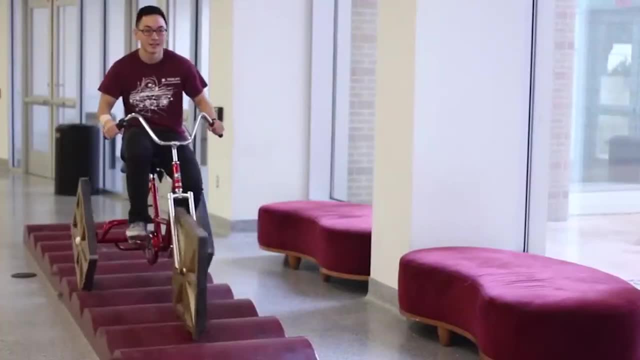 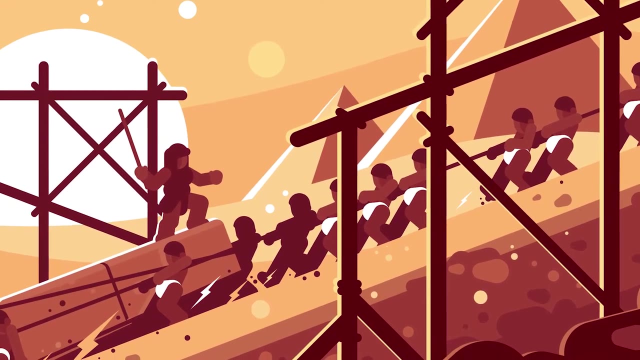 With the axle. the wheel could be attached on the end and turn freely about the axle. The axle would support the load. Did you know? if you have a rounded surface, you could have square wheels. This might have been how Egyptians moved the large blocks of stone for the pyramids.